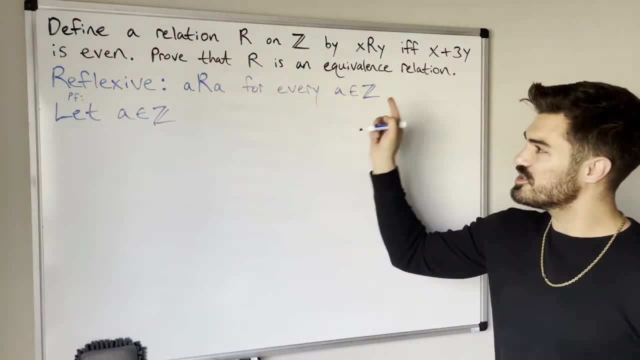 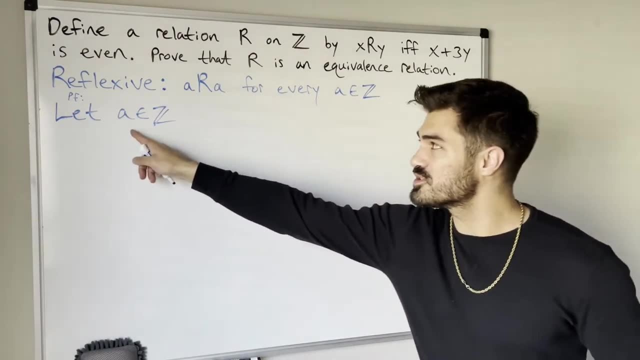 that here. Proof pf- right? This was just recalling the definition. Now we're starting the proof. So here's an arbitrary integer. What do we want to show about this integer? Well, we want to show that it's related to itself in this relation, right? So what does it mean for a to be related? 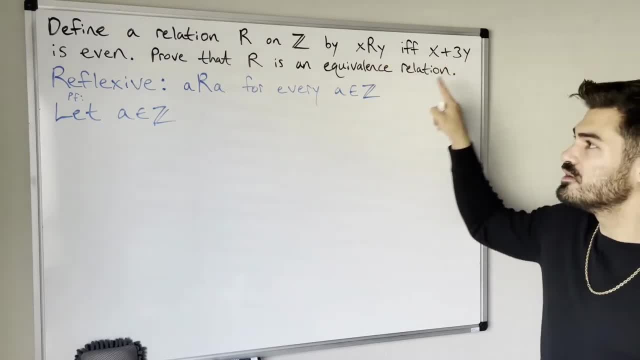 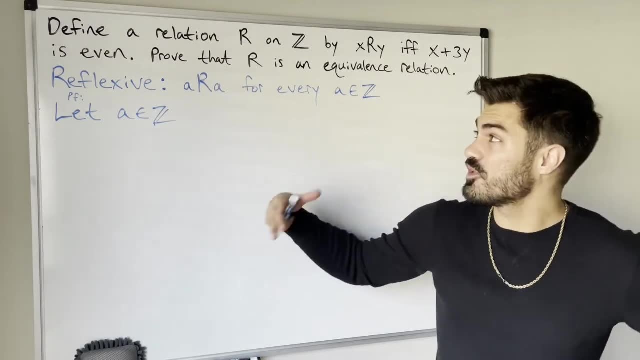 to itself. Well, that means that a plus three a is even. That's what would have to happen, right? So, really, what we want to show from here is that a plus three a is even, And then from that we can conclude, by the definition of this relation, that a is related to a. So we want to show 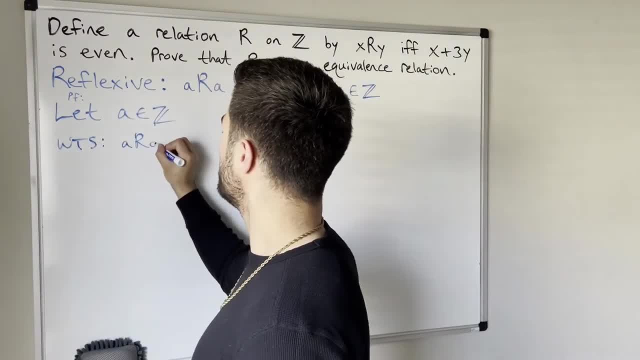 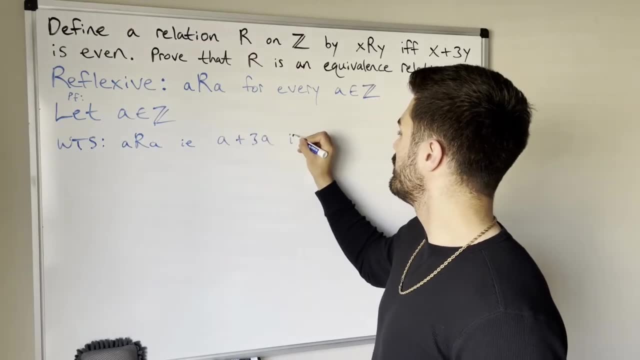 let's write that out. We want to show that a is related to a. In other words, we want to show that a plus three a is even. So what does it mean for an integer to be even? Okay, Well, to be even it means it could. 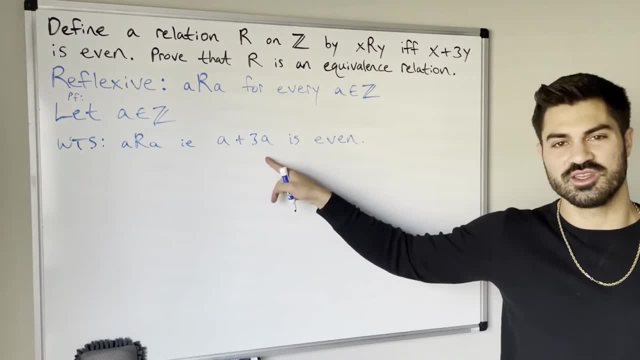 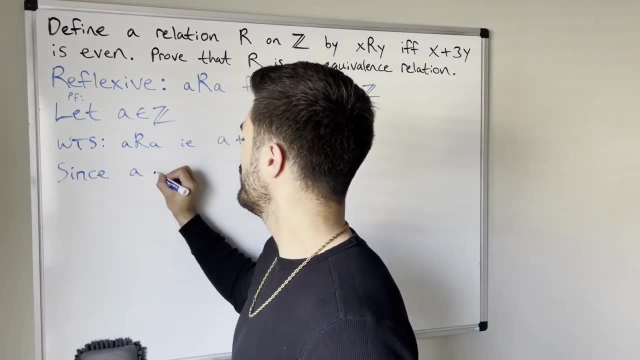 be written as two times an integer. So that's what we want to show about this, which actually isn't too difficult. We can actually probably do it in one line, Since a plus three a equals, we can just compute that. So we can just compute that. So we can just compute that. So we can just 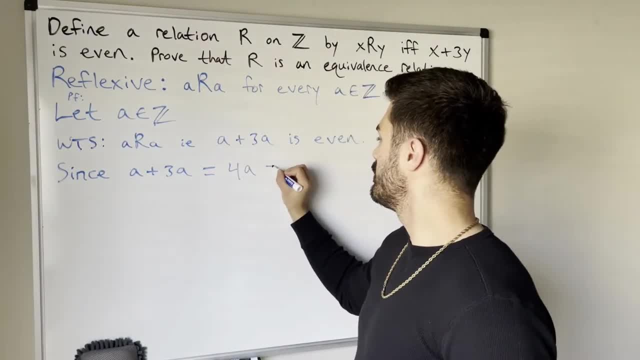 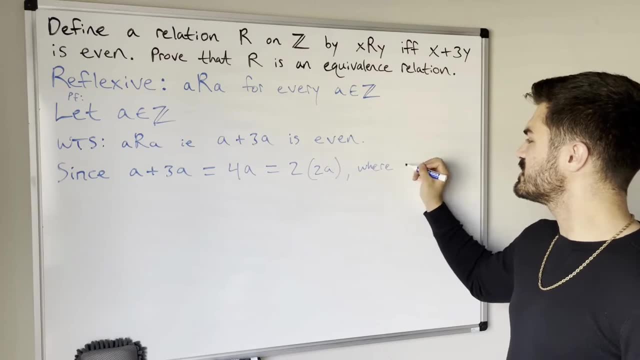 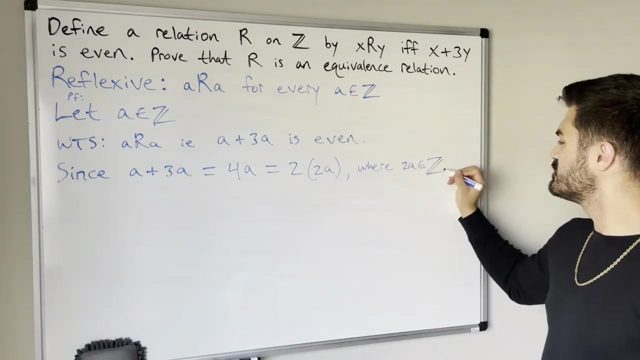 combine some like terms here: Four a, which equals two times two a, where two a is an integer, since a is an integer, right? If we take any integer and multiply it by two, we still get an integer. So two a is an integer. So what does this show? Since a plus three a equals four a. 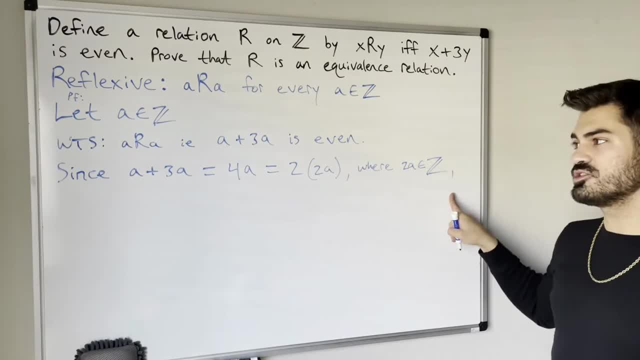 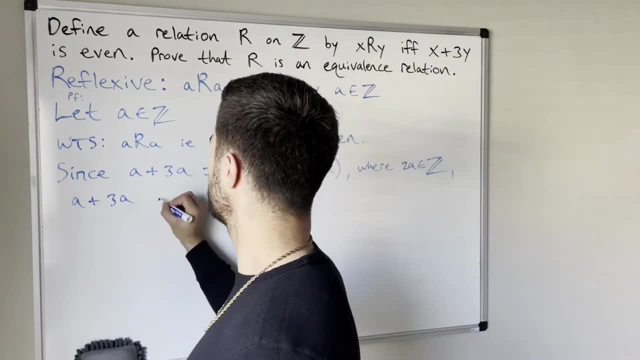 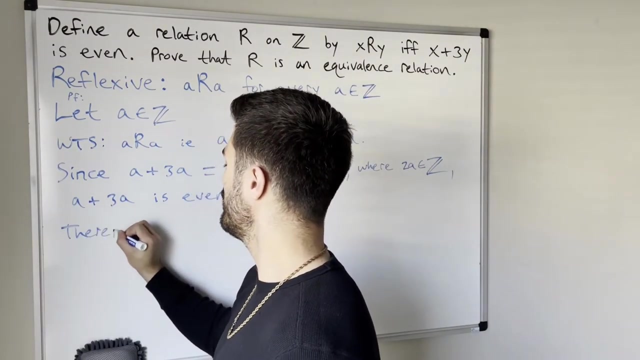 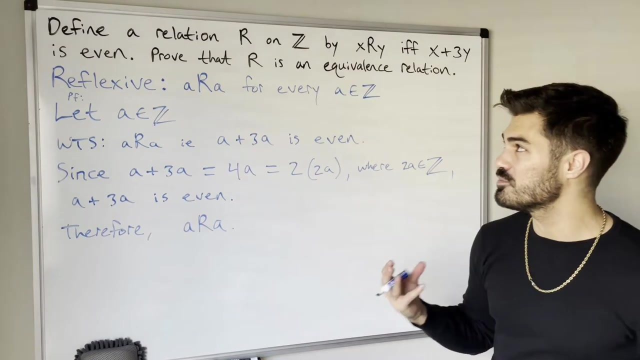 which equals two times two a, where two a is an integer. we know that a plus three a, a plus three a is even. Therefore, a is related to a. Hopefully, everyone sees the structure. This is essentially what we're going to do. anytime we're trying to prove a relation is reflexive. 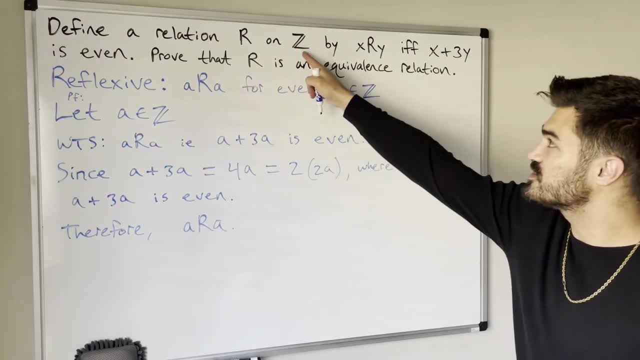 We're going to start with an arbitrary element in the set that the relation is defined on and we're going to try to show that that element is related to itself, which is going to be a little bit more difficult to do. So we're going to start with an arbitrary element in the set that 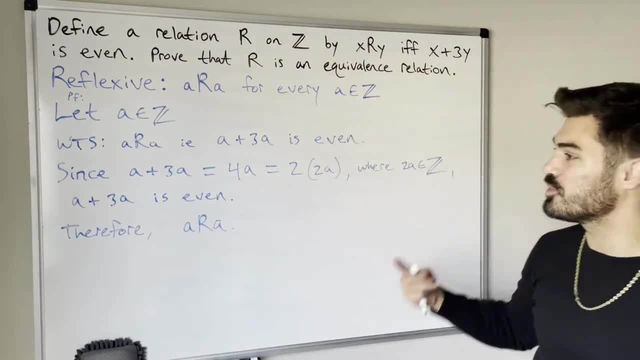 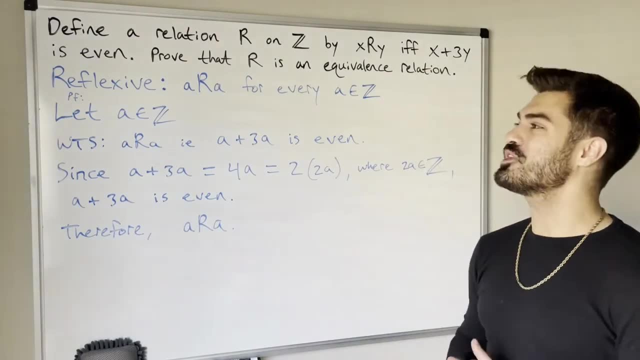 different depending on how the relation is defined. In this case, that meant that we wanted to show that a plus 3a was even, which we did pretty easily in a line, a line and a half. All right, let's see if we can prove that the relation is symmetric. now that we've shown that it's, 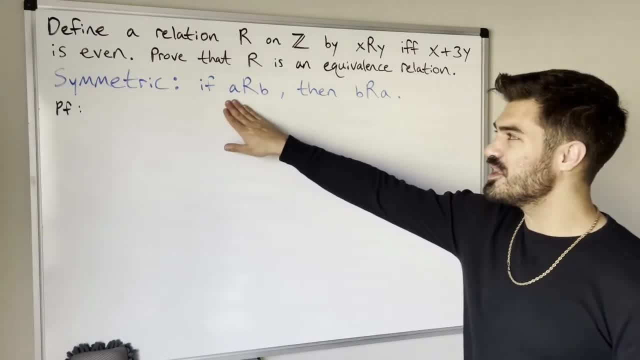 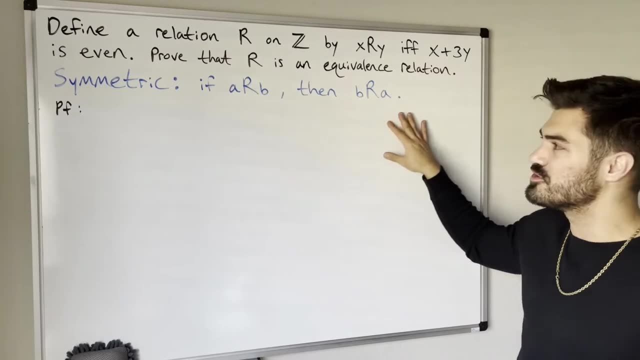 reflexive. So recall that symmetric means that if a is related to b, then b is related to a, and this is true for every a and b in this set of integers. So we have this sort of symmetry going on here, right? So how are we going to show that this relation is symmetric? 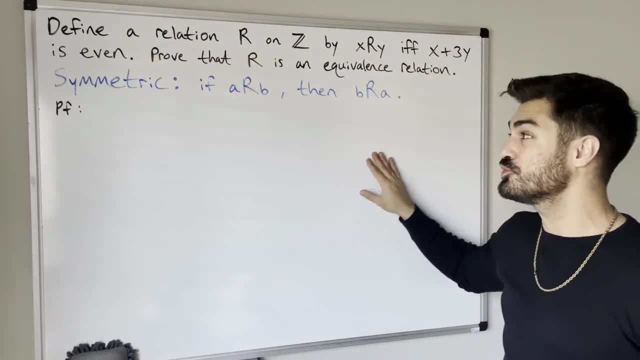 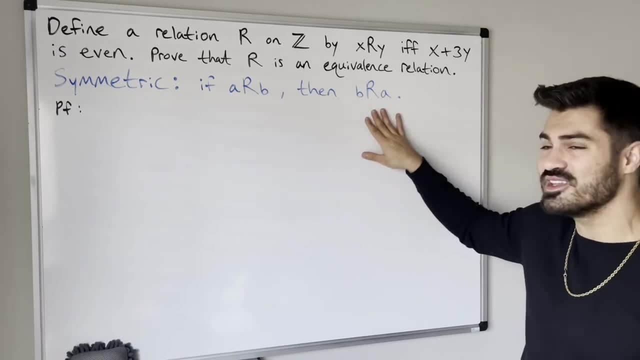 Well, this is a nice conditional statement. So we're going to use the direct proof method, where we assume that the if statement is true and try to show that that guarantees that the then statement is also true. okay, Direct proof method. So suppose that a is related to b. 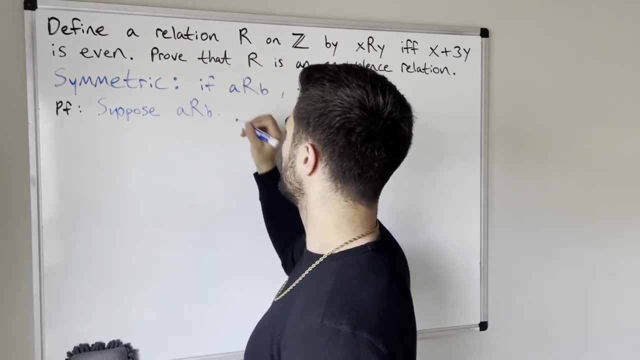 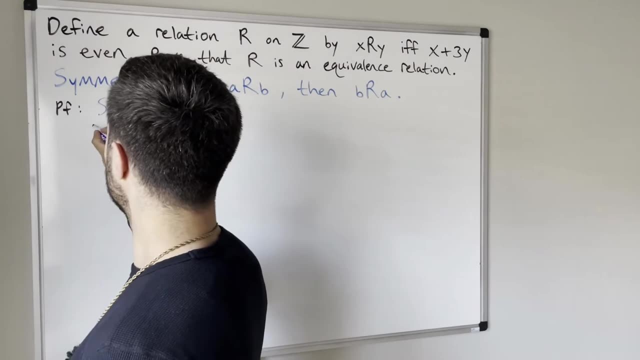 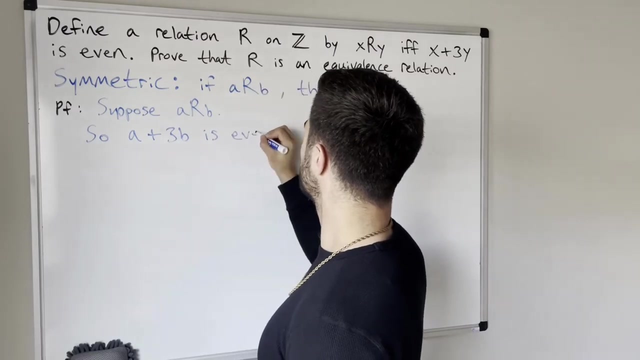 Suppose a is related to b. So what exactly does it mean for a to be symmetric? Well, that means that a plus 3 times b is even. So a plus 3 times b is even. And what does it mean for that to be even? Well, it means we can write that as 2 times an integer, right? 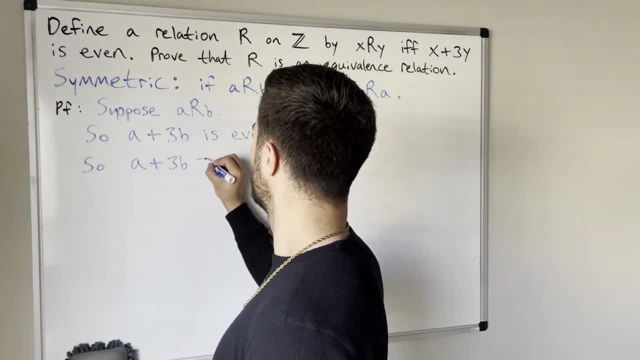 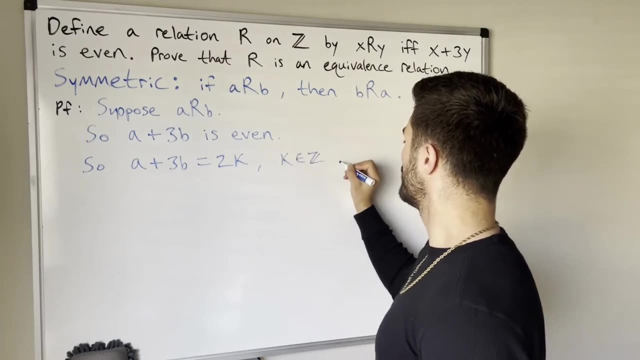 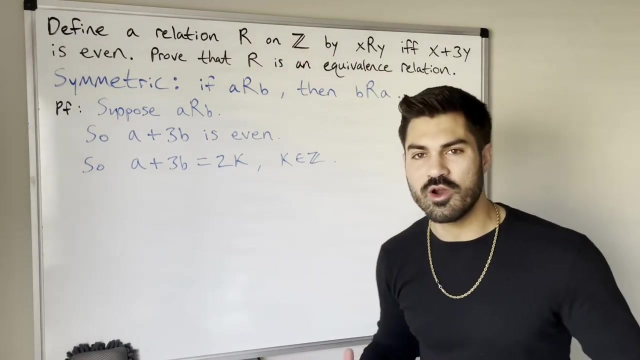 So a plus 3b equals, let's just call it 2k, where k is just some integer. okay, So that's what we got so far, just directly from our assumption, as well as how this relation is defined. So now let's think about what are we trying to show? Super important to think about what. 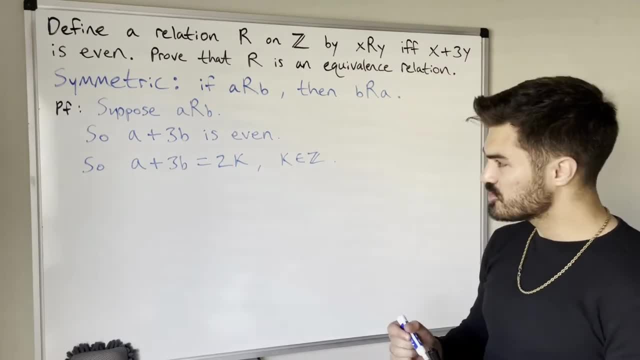 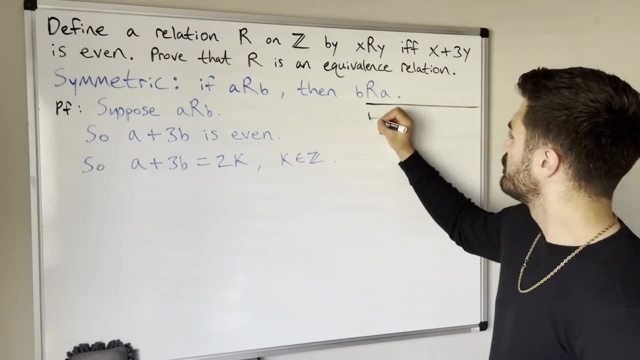 we're trying to show because we may have to do some scratch work, right? So maybe we'll do what we want to show off here to the side, okay, So I'll do a little box here for what we want to show. 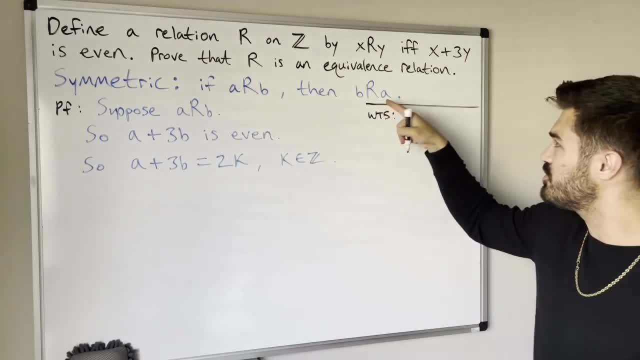 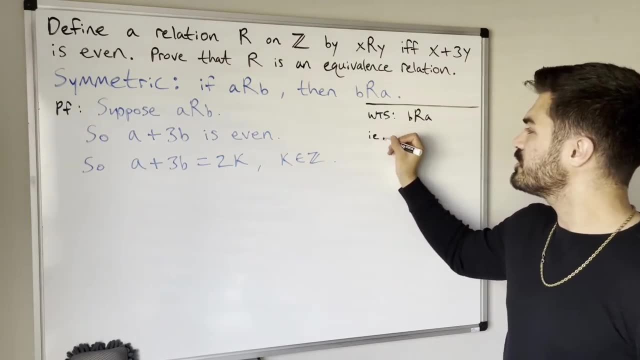 right, Because we want to assume that a is related to b and we want to show that b is related to a. and let's think about what this means. We want to show that b is related to a. In other words, we want to show that b plus 3a is even. 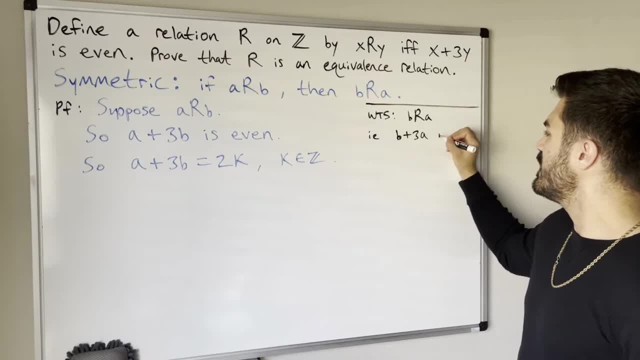 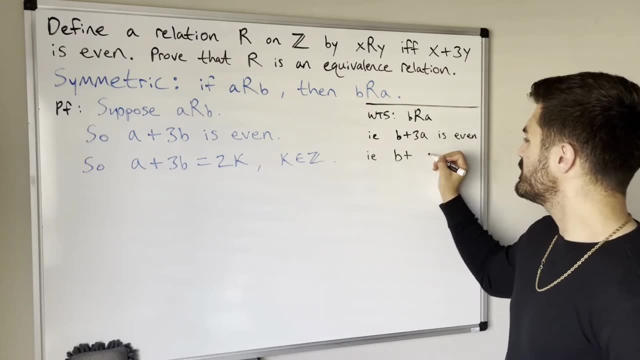 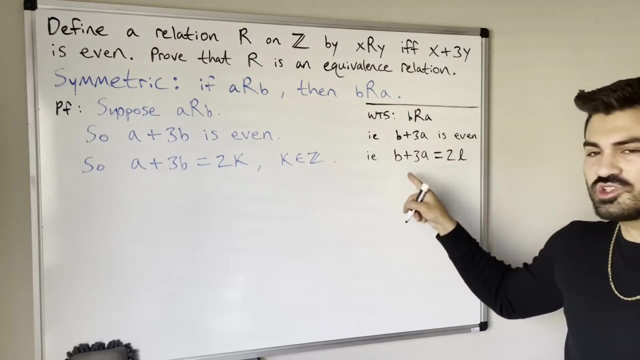 b plus 3a is even right, In other words that b plus 3a equals 2,. let's see, I already used k, so I'll use l right 2 times an integer. l is just some random integer, So now we got to think. 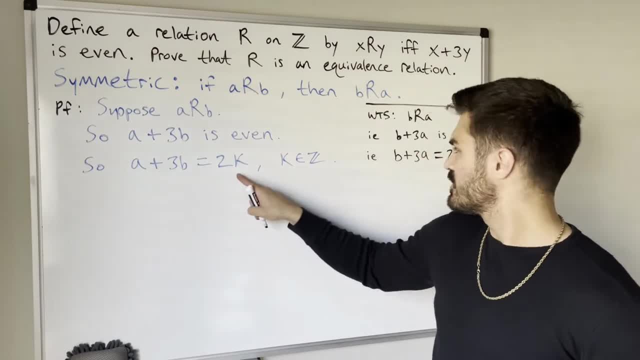 about. how can we use this to show that b is related to a And we want to show that b is related to a? This equation to show that b plus 3a equals 2 times an integer, and that's where our scratch work. 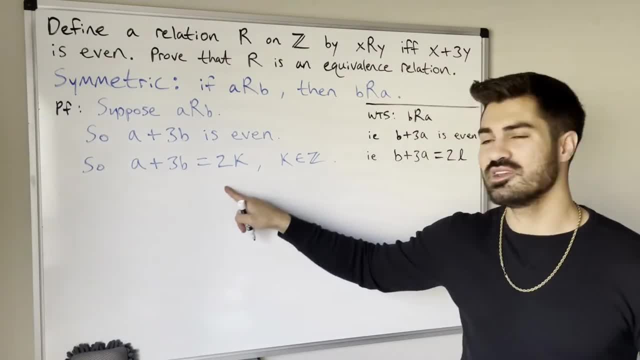 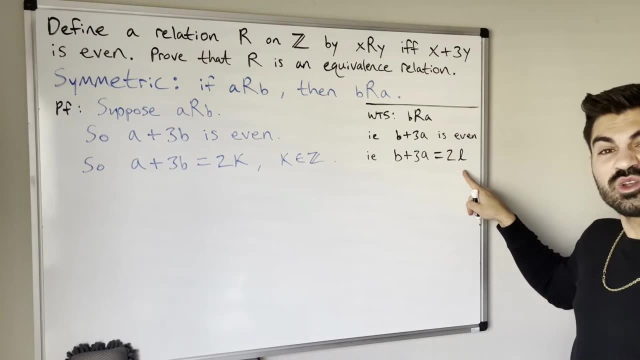 comes in, You can pull out an extra piece of paper, manipulate this, play around with this. So, if you want to pause the video and try that and see if you can get from this to this, and remember that l isn't going to literally be l, it's going to be just some integer, That's all it has to be. 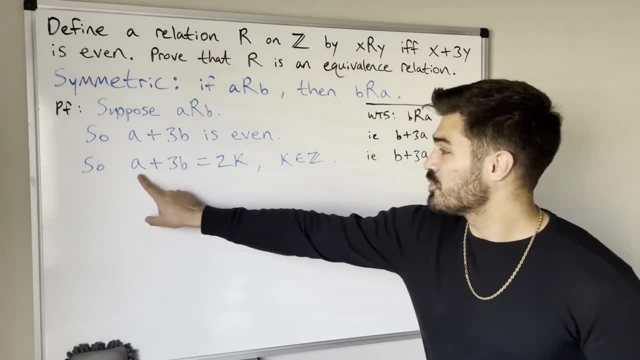 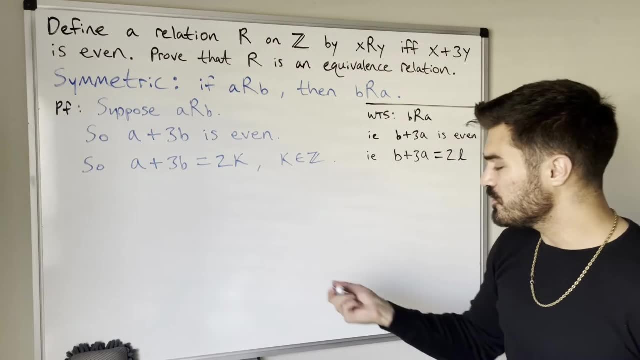 So here's what I did. I did a little scratch work and I noticed that we have an a here and we have a 3a here, So maybe we can multiply both sides of this equation by 3, and that will help us. So first I'm going to use the community. 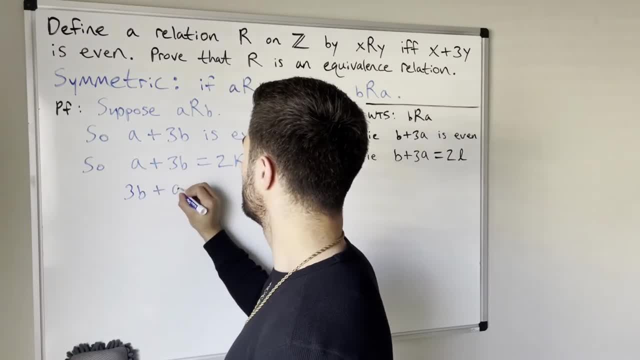 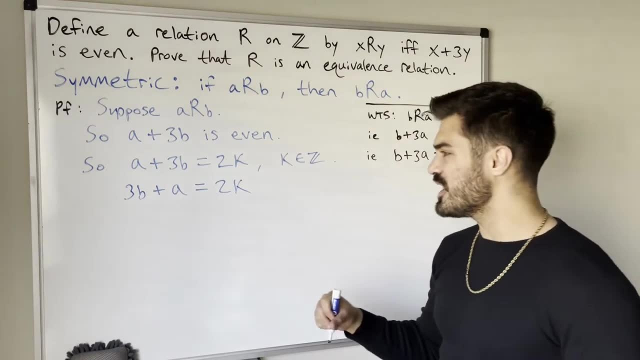 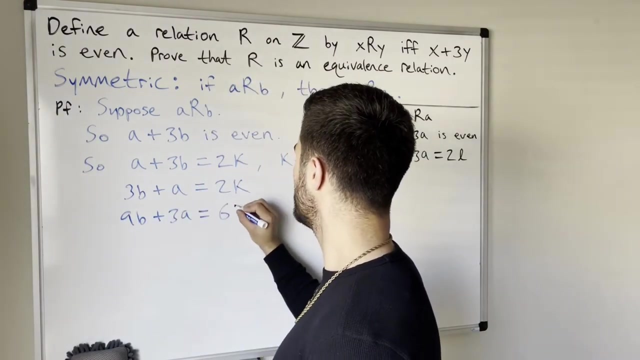 property. I'm going to switch the positions of these guys just so it better lines up with what I want to show. right, We have the b term first, a term second, so we can do that Now. let's multiply both sides by 3. We get 9b plus 3a equals 6k, where k is still some integer. 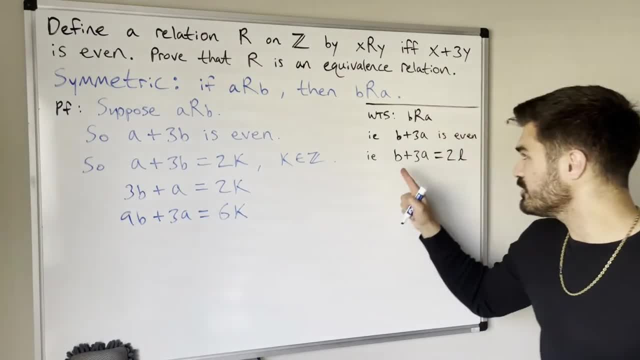 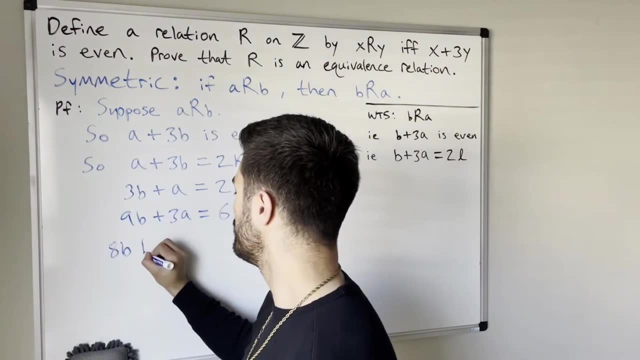 So we have our 3a, we're good to go. but now we have 9b And we really just want b. So maybe we can split this up and write 9b as 8b plus b, right, That's. 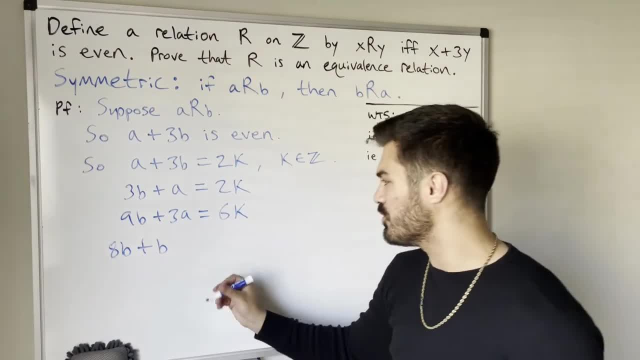 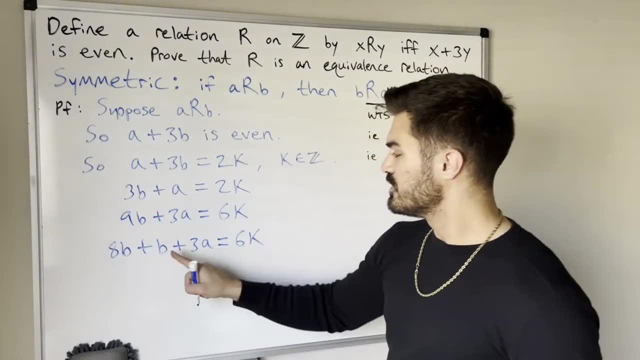 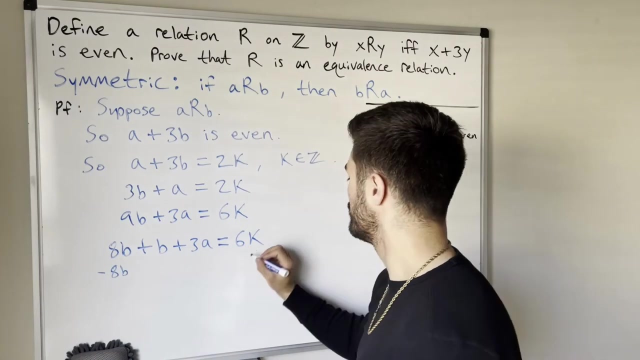 the same thing as 9b, 8b plus b, and now we have the b that we want here plus 3a, which equals 6k. So let's isolate this b plus 3a, and we can do that by subtracting 8b from both sides, right. 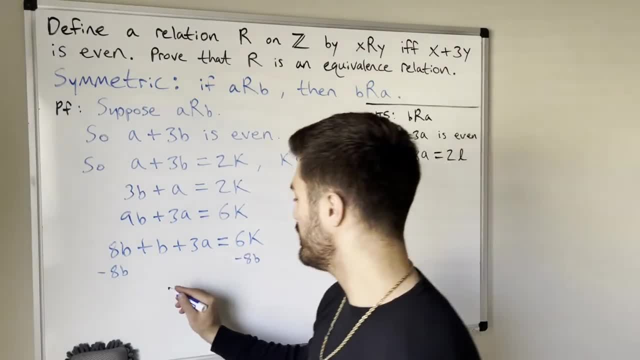 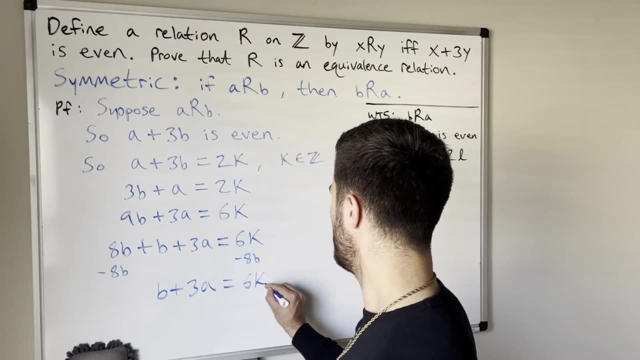 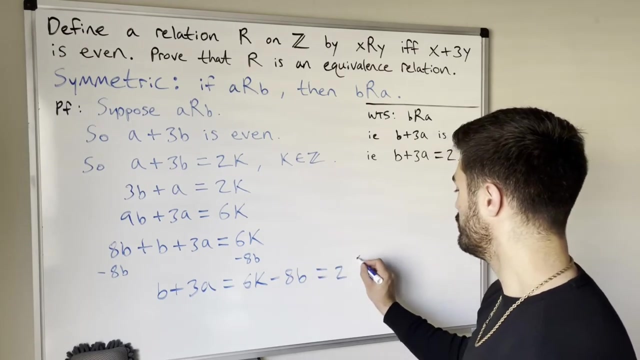 Minus 8b. So what we're left with here is that b plus 3a equals 6k minus 8b. We can factor out a 2 here, Factor out a 2, and we're left with 3k minus 4b. 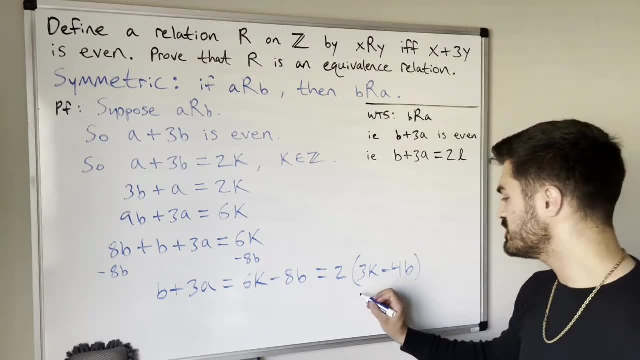 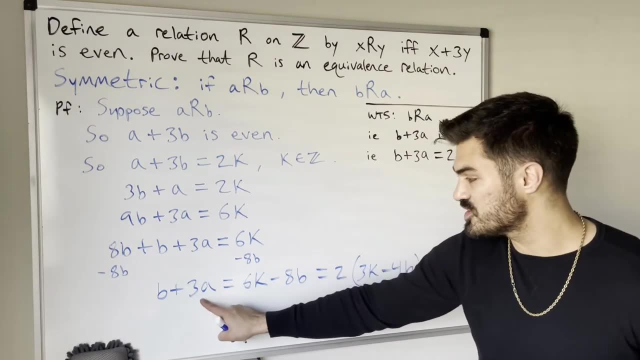 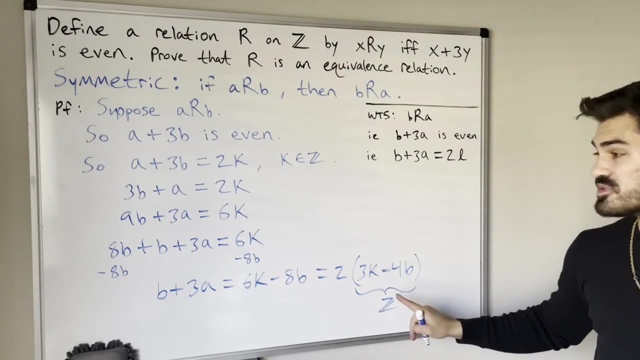 3 times an integer minus 4 times an integer, Which means that we can write: b plus 3a is 2 times an integer, which is exactly what we wanted to show: That b plus 3a is 2 times an integer. okay. 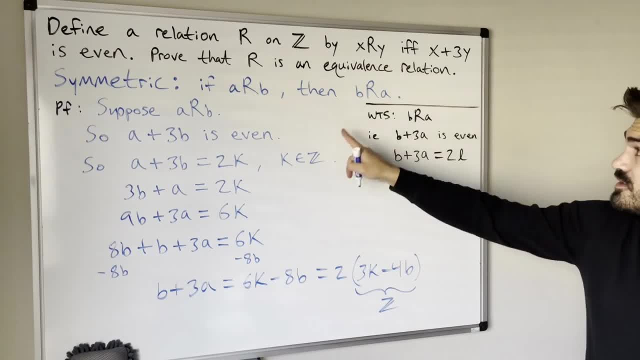 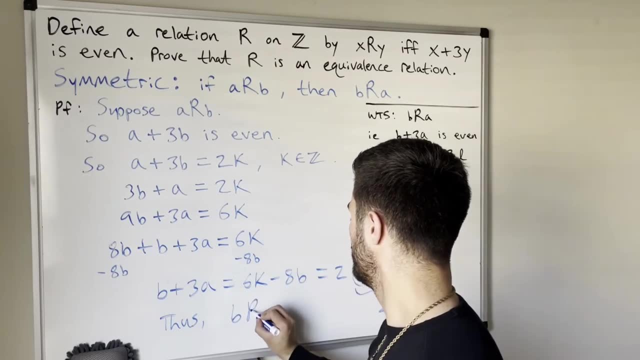 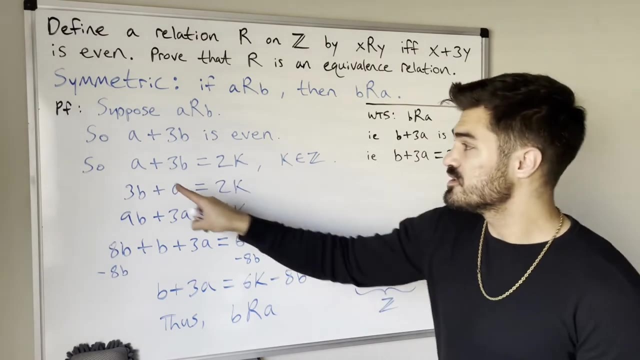 And that's really it. Therefore, b is related to a. Thus b is related to a. So again, you can do some scratch work. You can even work backwards, Start with this and manipulate this To see if you can get to this right. 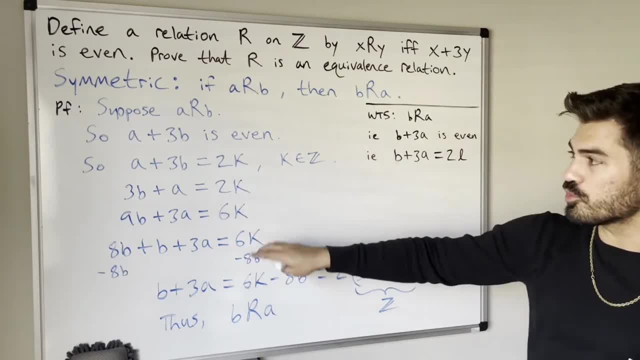 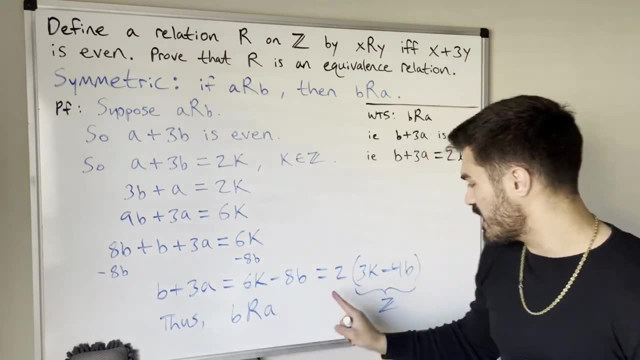 As long as all of that is in your scratch work. At the end, once you write out the formal proof, you want to start from your assumption, from what you know, and you want to move toward what you want to show, which is that b plus 3a equals 2 times an integer. 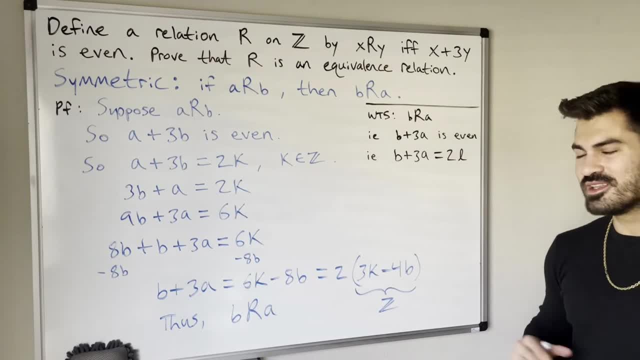 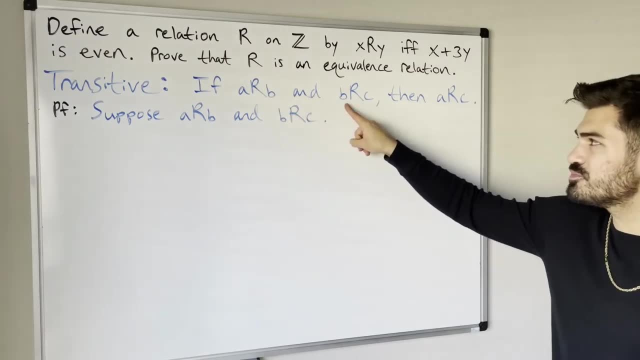 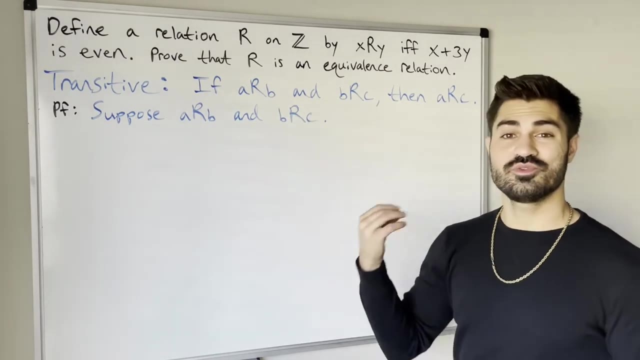 Therefore b is related to a. Let's see if we can prove that this relation is transitive. So recall that transitive means that if a is related to b and b is related to c, then a is related to c. So how we can show this is again the direct proof method. 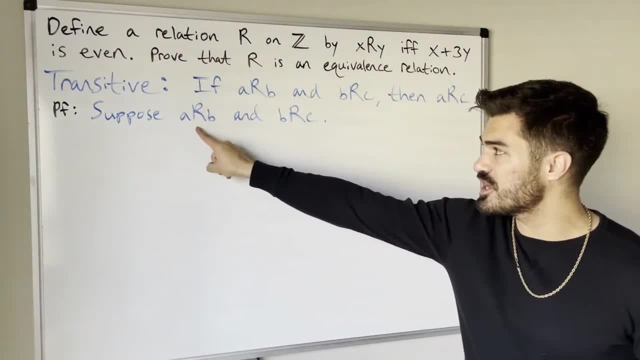 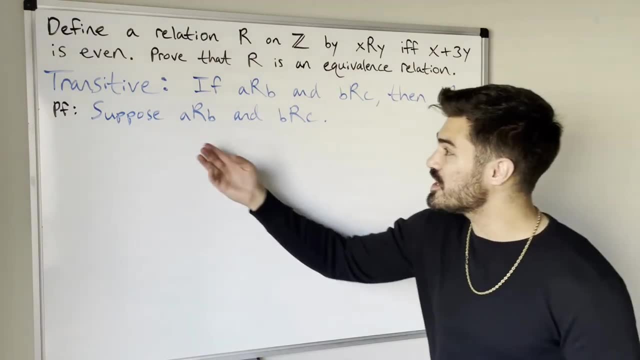 We're going to assume this, if statement is true. So suppose a is related to b and b is related to c, And what we want to show is that a is related to c. So what can we say from this assumption That a is related to b and b is related to c? 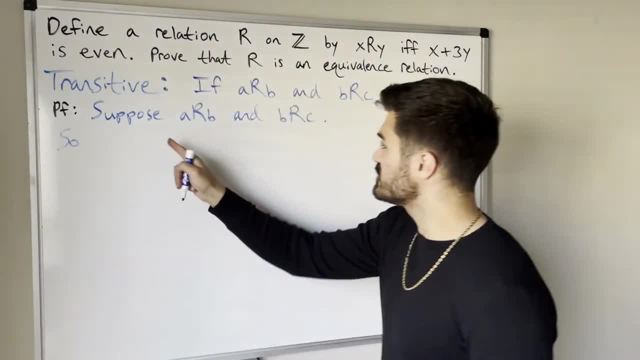 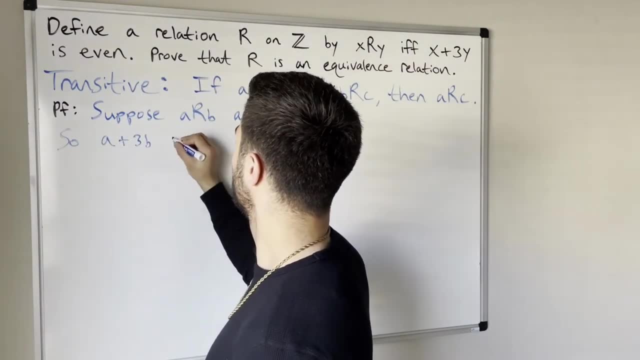 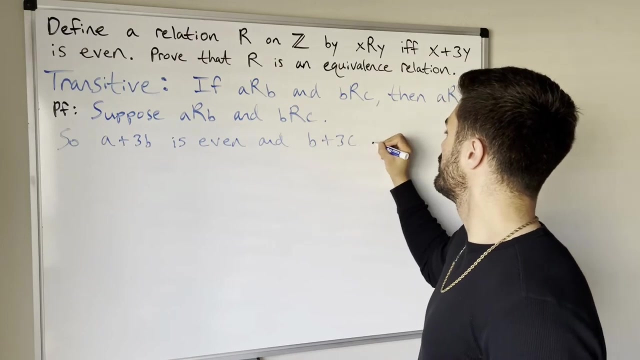 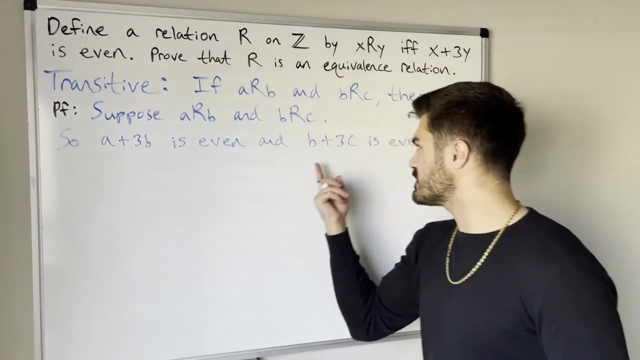 Well then I'll say so: a plus 3b is even, a plus 3b Is even, And b plus 3c is even. And what does it mean? What is the definition of even? Well, both of these can be written as 2 times an integer right. 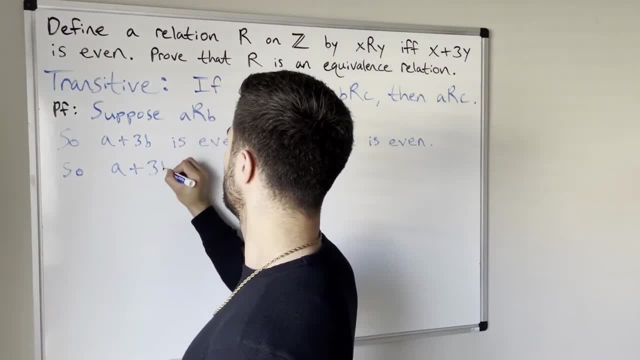 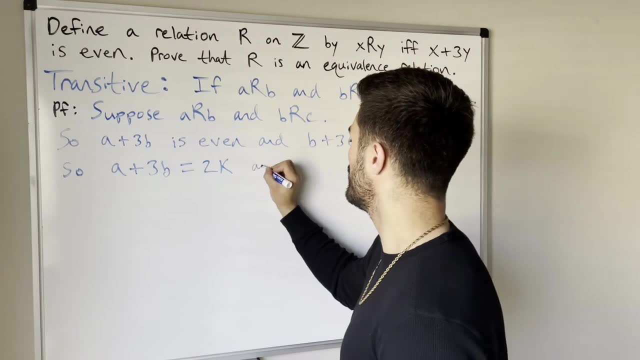 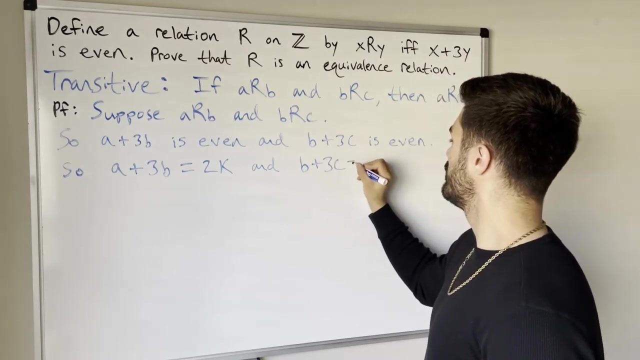 So a plus 3b equals 2.. We'll use k for this one and we'll use l for this one, okay? So a plus 3b, 3b equals 2k, And b plus 3c equals 2l, where k and l are both integers. 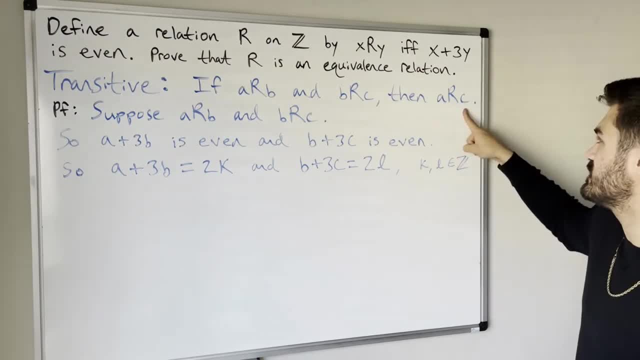 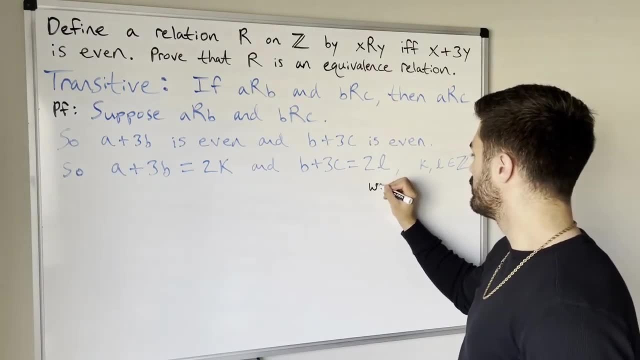 So now let's think about what we want to show. We want to show that a is related to c, In other words, that a plus 3c is even So. let's do that off to the side. here again Want to show that a is related to c. 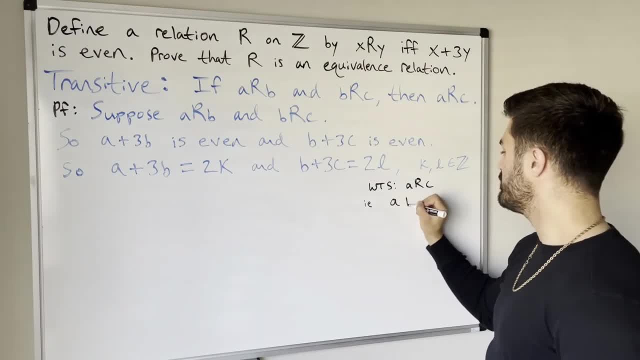 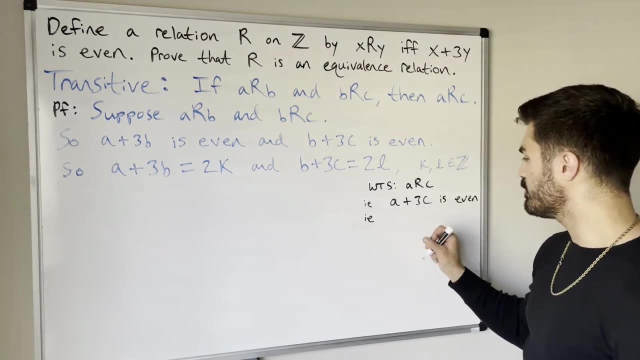 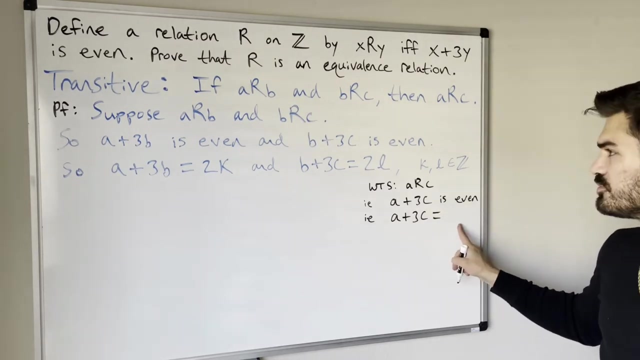 What exactly does this mean? Well, that means that a plus 3c is even, And by the definition of even, let's get even more precise- that a plus 3c equals 2 times an integer. We've already used k. 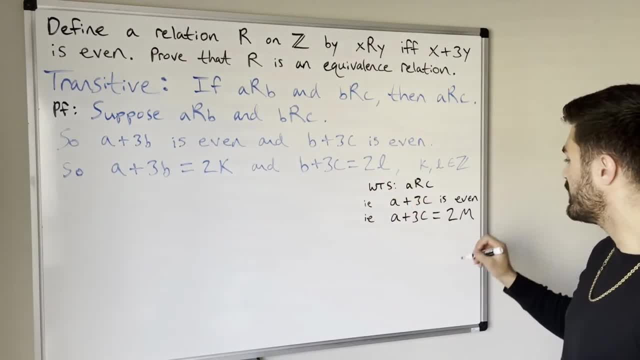 We've used l, so let's use m 2 times m, Right? So this is what we want to show, And again we can kind of use this play around with it, but I really like to write this out and keep it in mind. 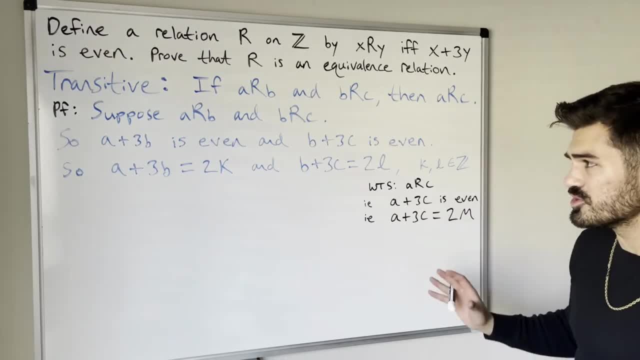 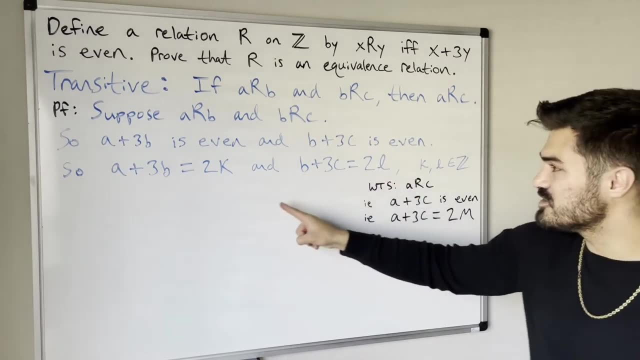 Really important, when we're first learning how to do proofs, that we think about what we want to show, so we can think about how we're going to get there. So what I notice here is that I think I can combine these two equations Right. 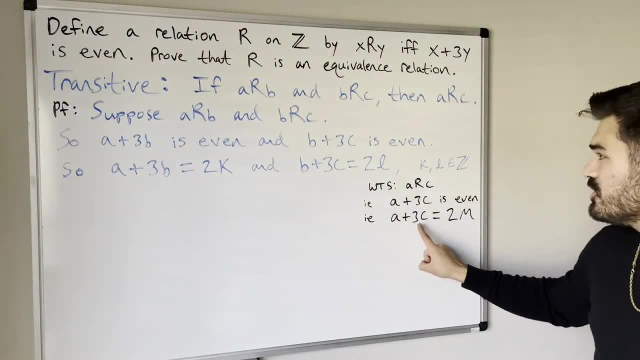 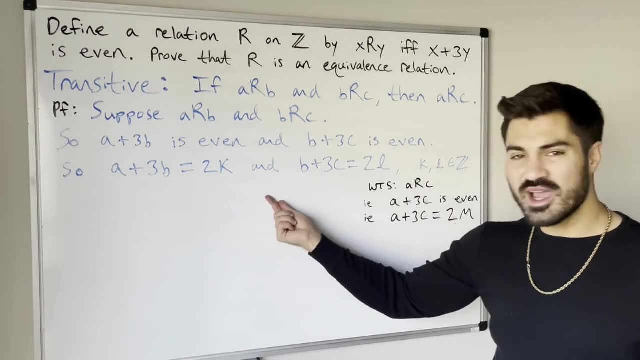 I can add these two equations together, because what I notice is that this one has an a, which I need here, and this one has a 3c, which I need here. So maybe if I combine these right- Because if a plus 3b equals 2k- 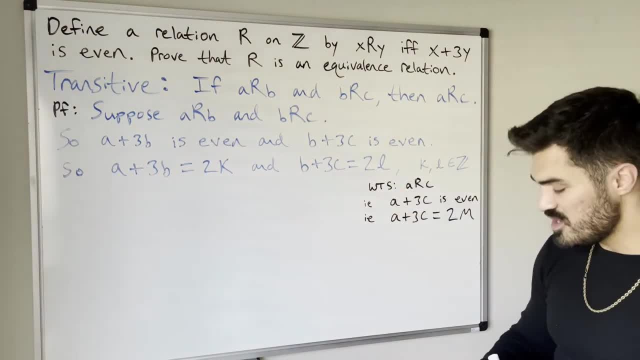 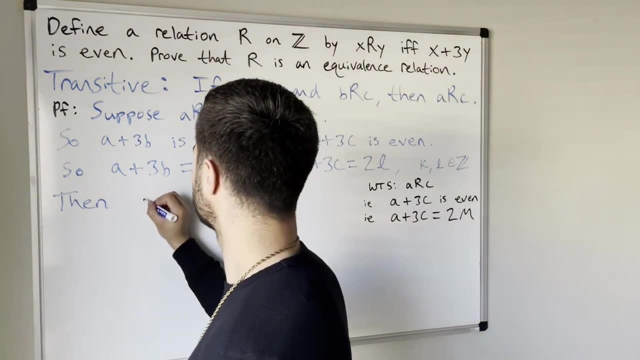 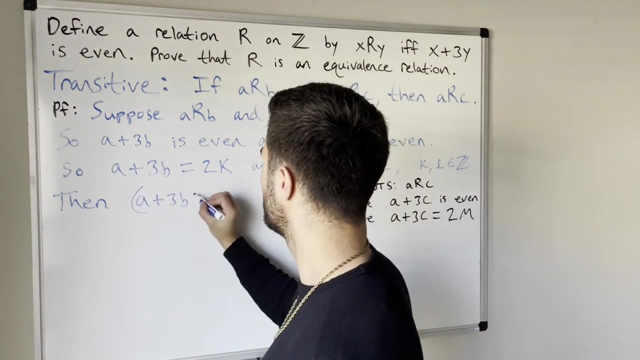 and b plus 3c equals 2l. then what we have is that a plus 3b plus b plus 3c- and I should technically use parentheses here, although I'm going to end up not needing them, But I'll do it to emphasize what I'm doing here. 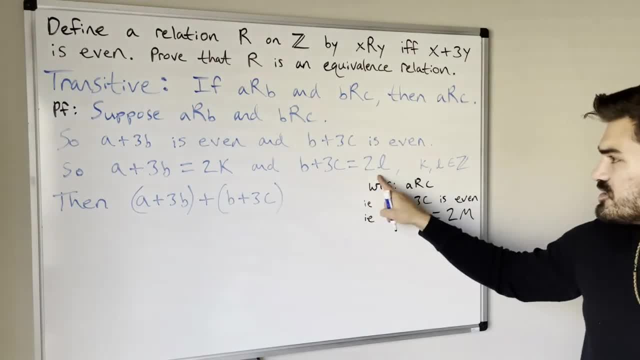 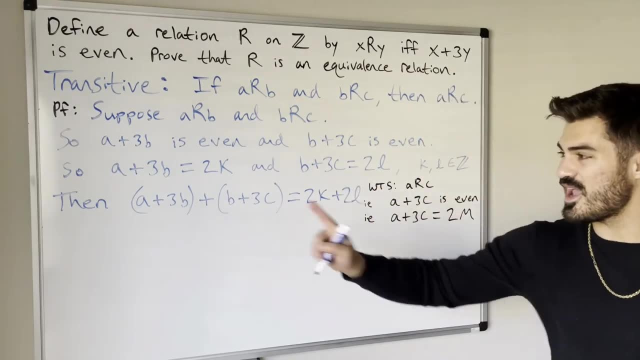 Right, If I add this plus this, then I should get this plus this: 2k plus 2l. 2k plus 2l. Okay, So adding these two together Now. we don't need the parentheses, Obviously. 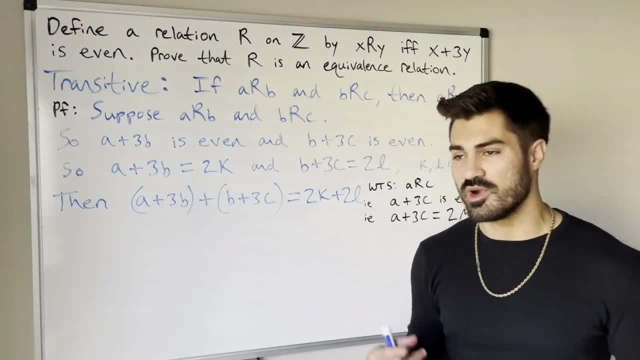 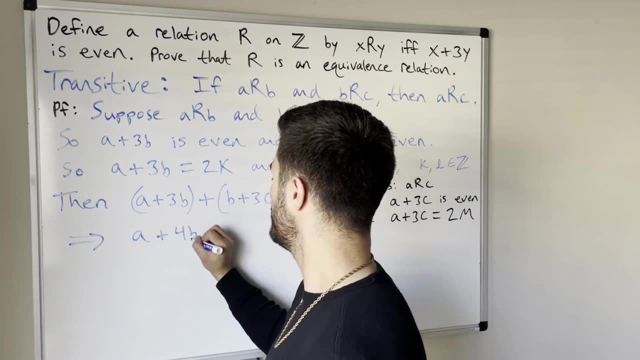 we can get rid of them and we can combine some like terms: 3b plus b. we can write that as 4b, Right? So this- I'll just draw an arrow- gives us a plus 4b plus 3c equals 2k plus 2l. 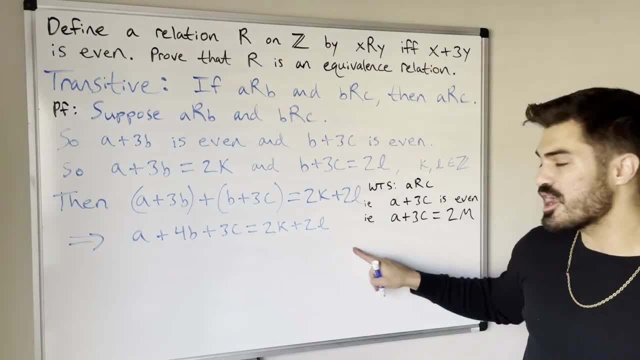 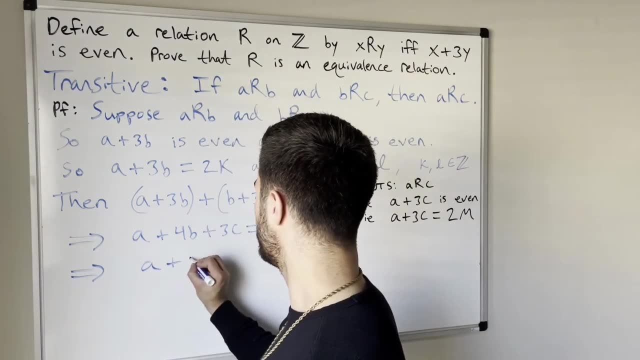 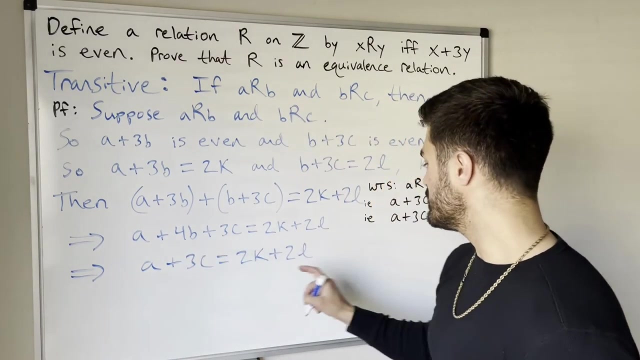 Okay, So now we're so close. Really, all we need to do is subtract 4b from both sides, So another arrow here, Right? This implies that a plus 3c equals 2k plus 2l minus 4b. 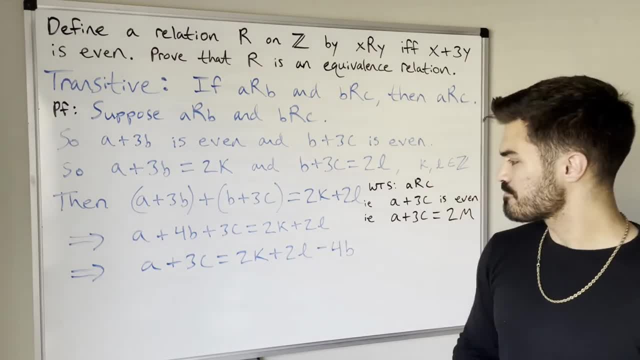 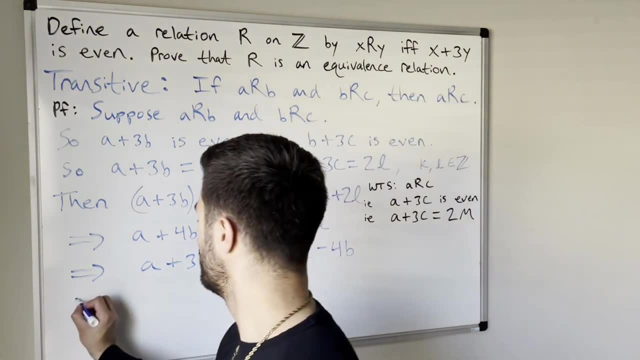 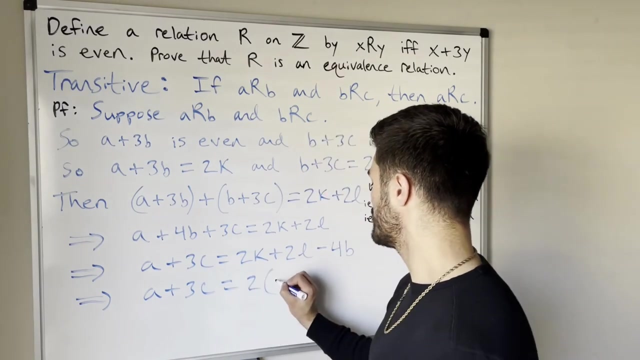 I subtracted that from both sides, I just didn't write out the step. I think we can do this now. We can factor out a 2. Right From this entire right hand side of the equation. So a plus 3c equals 2 times k plus l minus 4b. 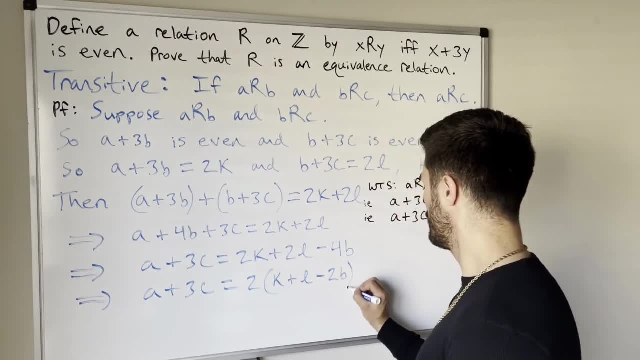 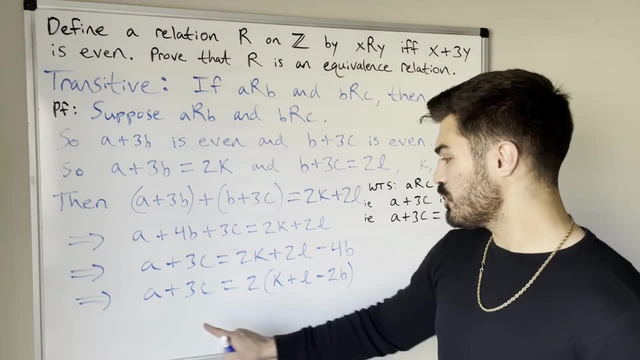 Okay, minus 2b, This whole thing is an integer. k is l is, b is right. Whole thing is an integer. So what we've shown is that a plus 3c equals 2 times some integer. So in this case, this thing here is: 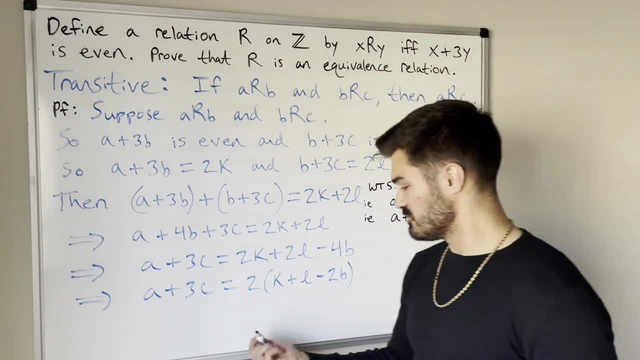 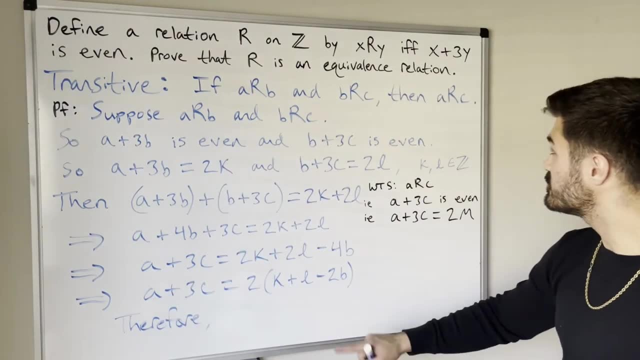 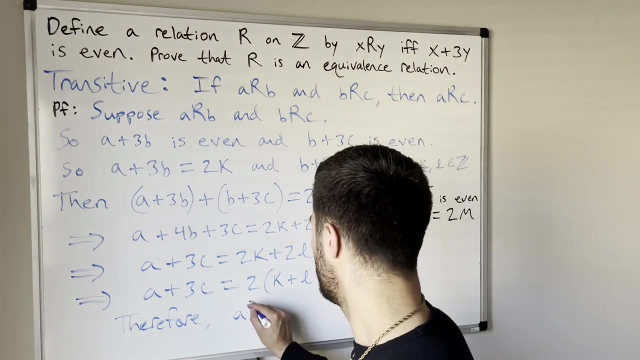 our m right, Some integer And therefore we've done right, We're done. Therefore, what a is related to c? because a plus 3c is 2 times an integer or even right, So a is related. 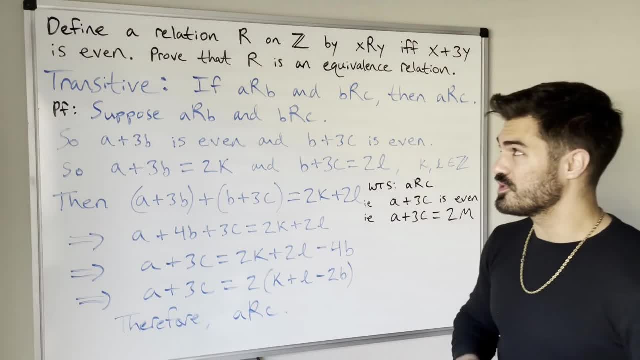 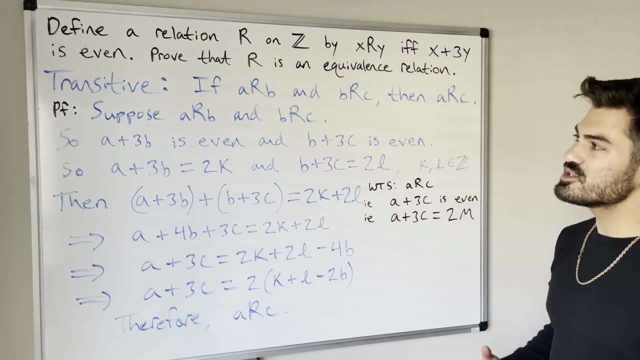 to c. So this is the general structure for how we're going to prove that a relation is an equivalence relation. We're going to go through reflexive, symmetric, transitive, and the general structure of each of these proofs for each of these properties pretty much stays the same. We're 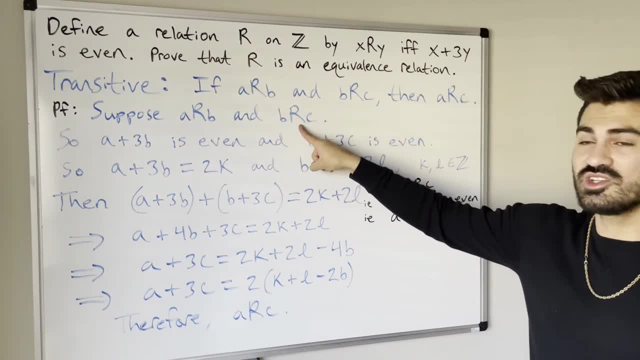 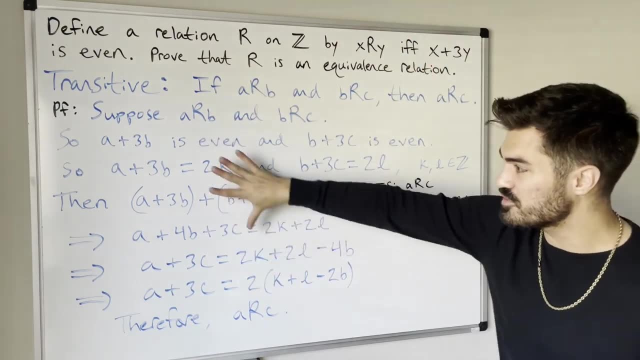 always going to suppose that a is related to b and b is related to c And we're always going to try to show that this means that a is related to c. It's just depending on how the relation is defined. the stuff that goes on in the middle may be a little bit different, But the general 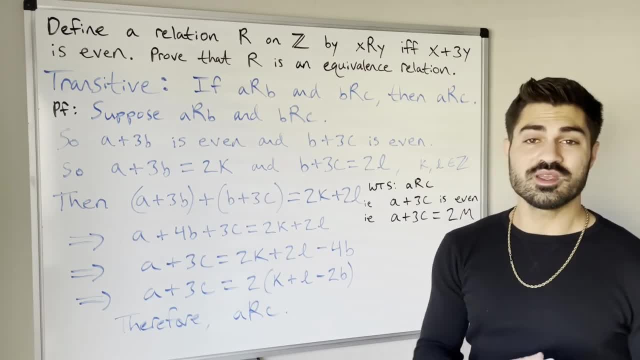 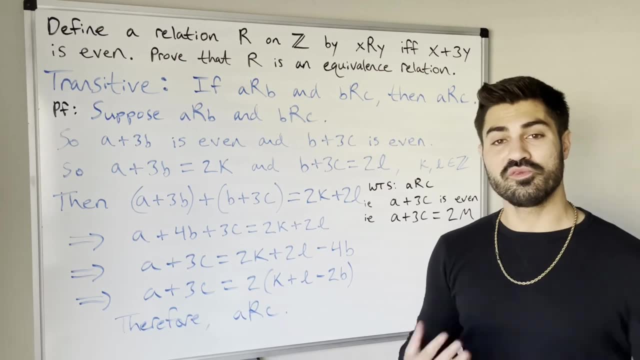 structure is the same. When we're starting with reflexive, we always let there be an arbitrary element in the set the relation is defined on And then we try to show that it's related to itself. And with reflexive, we always start that assuming a is related to b and trying to show that b is. 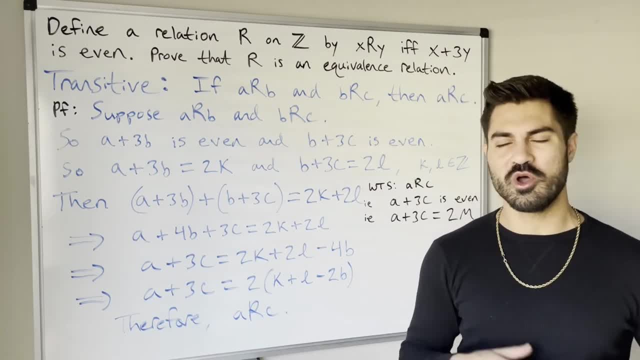 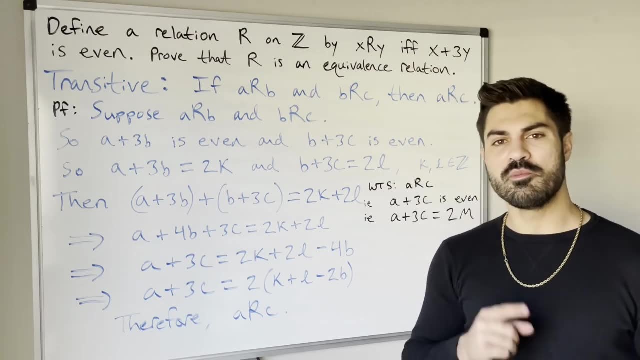 related to a, So maybe I'll do one more example and upload it on this channel, But hopefully this helps. If you have any comments, questions, anything, feedback, leave it below. Hit like, hit, subscribe. But, most importantly, keep flexing those brain muscles and I'll see y'all later.